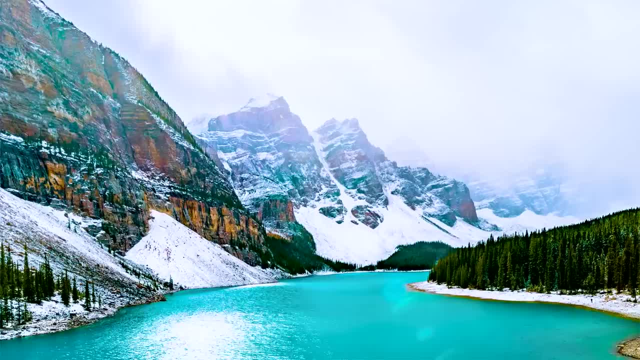 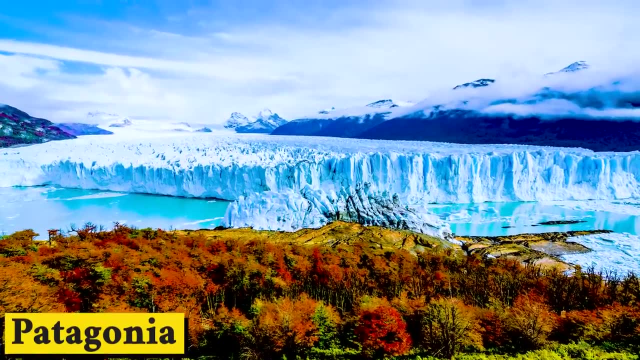 In summer, it's the best time. If you want to go to the United States or Canada in summer, it's the best time. Or if you want to check the glaciers down in Patagonia in Latin America, the summer is the best time. So you have one of those times, those three months, June, July. 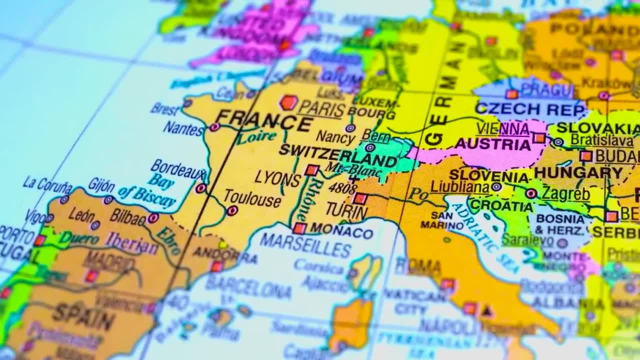 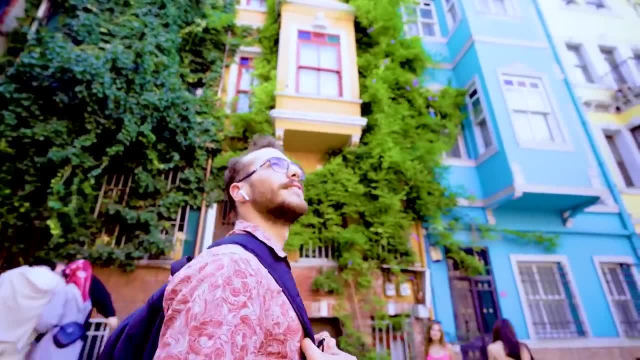 and August, where you can go and explore other places around the world, which is exactly what I did last year, 2022.. 2021 is when I spent all summer here, 2022,. I did a lot of traveling during summer. I was not here at all, And that's what I recommend a lot of my clients If it's possible. 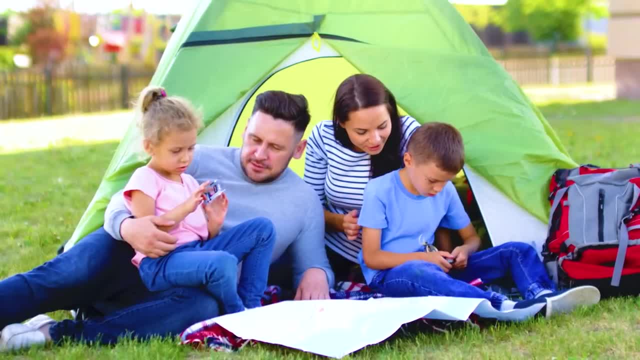 for you, obviously, if you have kids, if you have a wife, if you, for example, your wife has a job here in Dubai, or you have things tying you here, or you don't want to go anywhere else, you just 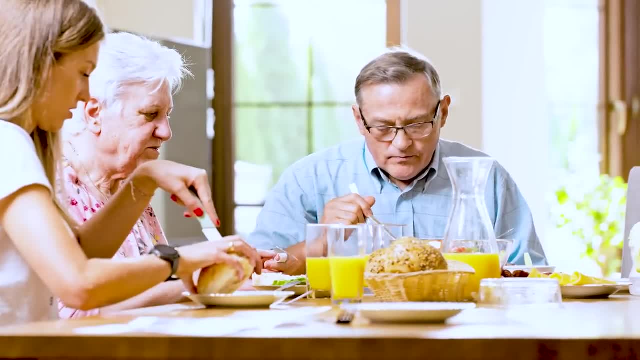 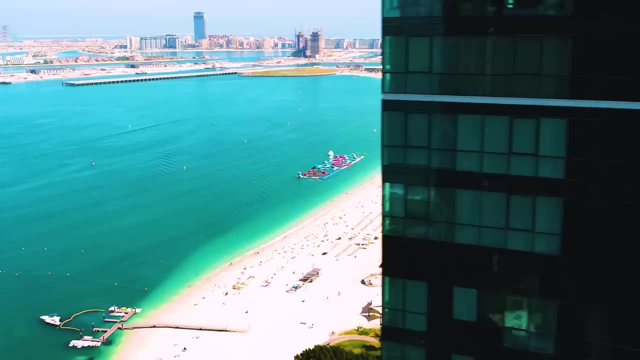 want to take care of your parents. anything you want to do That summer, it's still bearable. You can still lift through it. It's not you're going to die or burn outside A lot of locals. what they do is they just go to the mall. They go to the beach very early in the morning or late in the 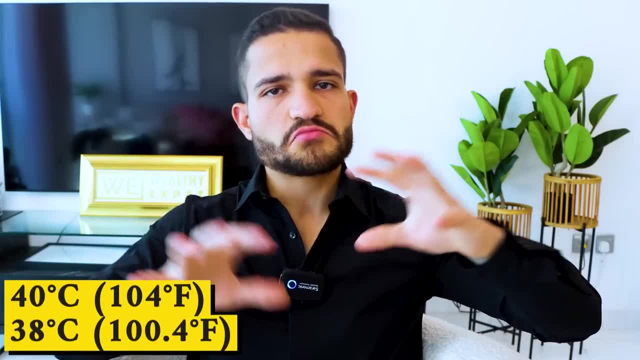 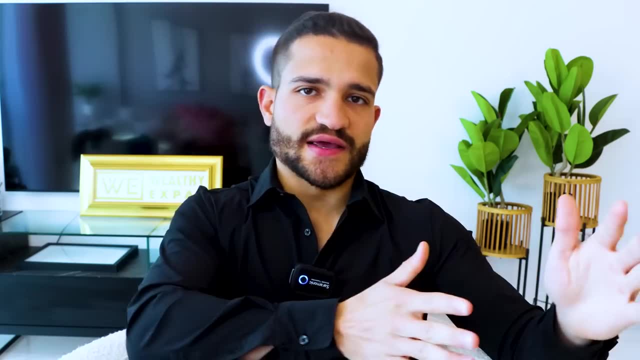 evening, because in the evening the temperature drops to about 40,, 38,- I would say around that range, And it's not that bad. It's still very hot, but it's not as bad as during the day. So you can. 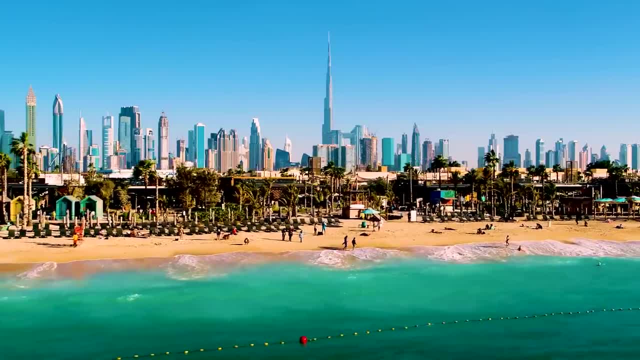 still live a regular life. You just can go to the beach, go outside in the morning and in the evening, And during the day you want to go to the mall, be in your car in AC, or in an Uber with AC, or in your apartment with. 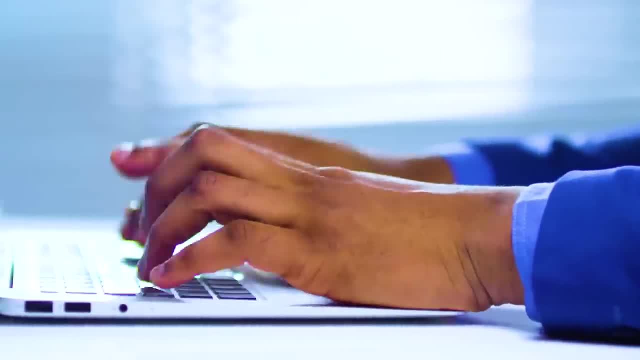 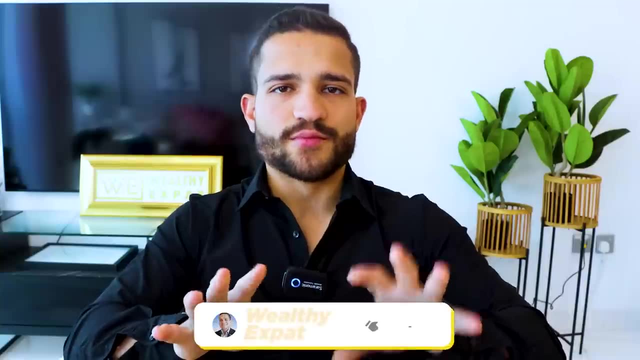 AC And you can focus and hustle and work as well. If you're trying to work harder on your computer or for longer hours, the summer is perfect, because you go outside and you want to come back in and keep working. So that's what I remember from August of 2021. It was horrible to be outside. 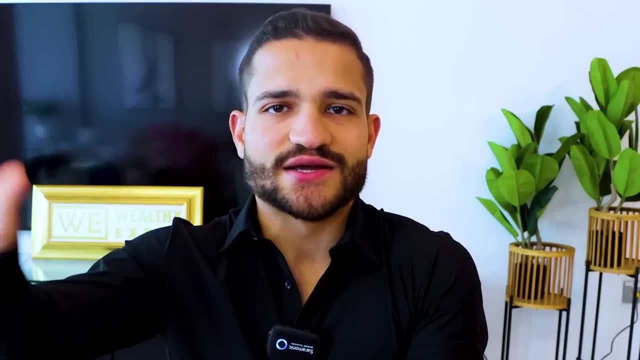 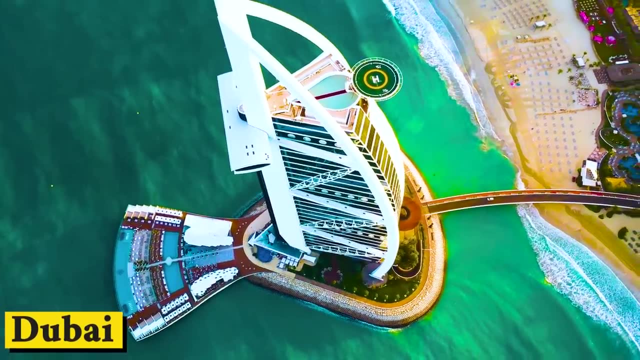 but I was always at home working because I was more focused, because outside you just can't go. What do you think about the weather in Dubai? Is it too extreme, Is the heat just too much and makes it an unbearable place to live, Or is it fine? You just go out in the summer, come back in? 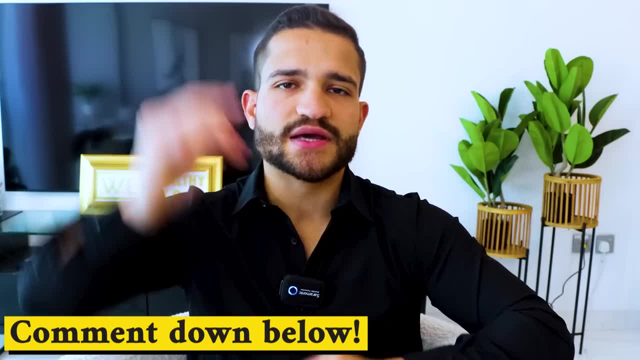 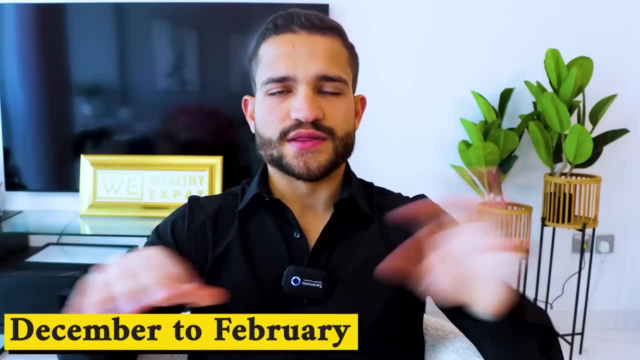 the winter and you split your time between different places. Let me know your opinion in the comments below. The best months to be in Dubai is right now when I'm making this video: December to February. These three months- anything from the end of October, start of November, all the